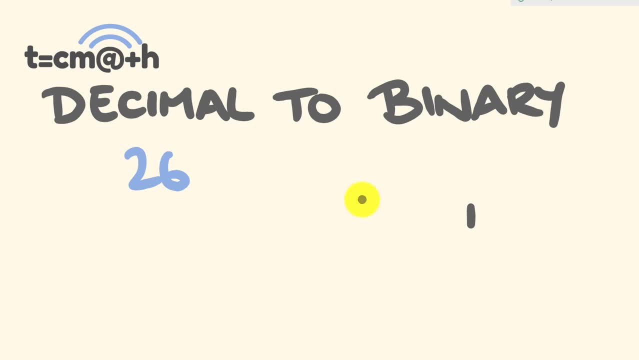 start on the right here And I'm going to start with a 1 and I'm going to start doubling this number. I'm going to keep doubling up until the doubling I get would exceed 26.. I'll show you what I mean. So 1,, 2, double of 2 is 4, double of 4 is 8, double of 8 is 16, and double of 16 is 32.. So 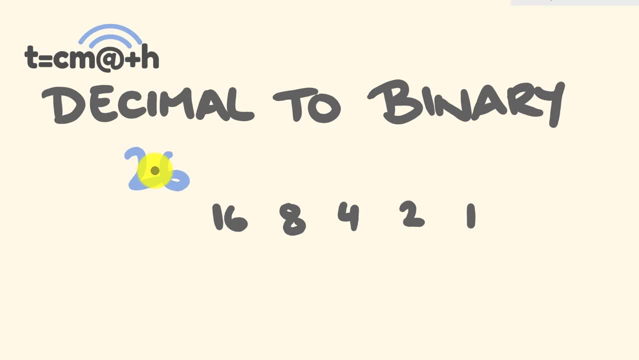 I don't need to go that far, because that would exceed 26.. That's the first step. The next thing is we're going to look at these numbers we have here and see what numbers we need to add to get 26.. So I'd start on 16 and I'd think, OK, 16 plus 8 is 24.. We will use that one as well. What number? 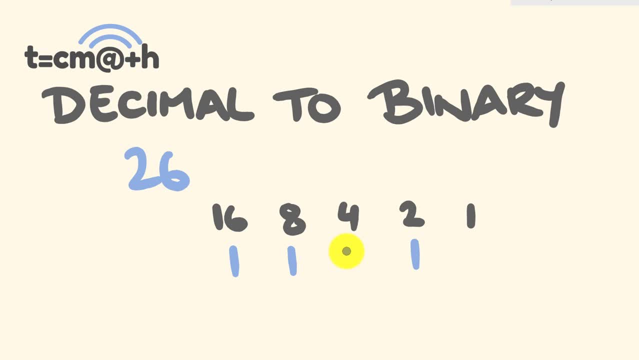 do we need to add to 24 to get 26?? And it's 2.. So these numbers are going to have zeros. The binary equivalent of 26 is 1, 1, 0, 1, 0.. What about? I give you a couple of examples. So why don't we? 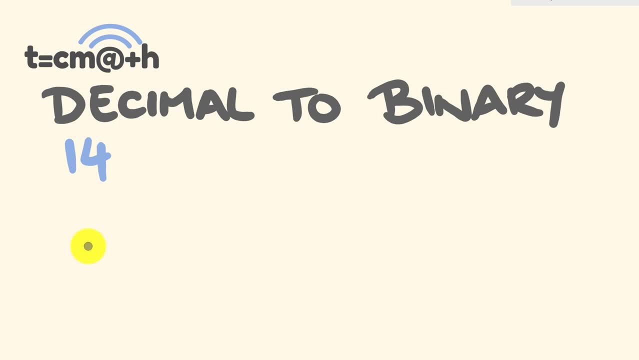 try to do decimal 14 across to its binary equivalent And 35 across to its binary equivalent. So the first thing we do is we're going to start on the right here and start doubling, So 1,, 2,, 4,, 8.. We don't need to go up to 16 because it would exceed. 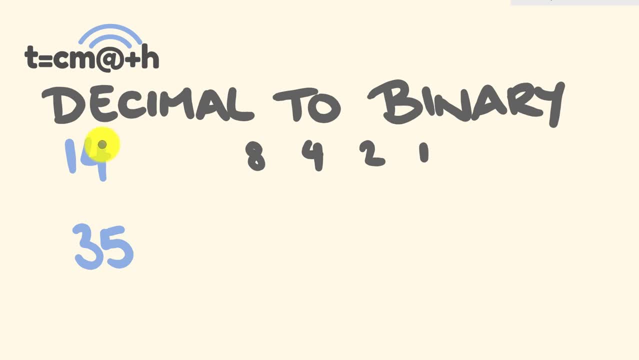 14.. Now we're looking at out of these numbers what we need to add to get 14.. OK, so 1 is going to go under the 8. here We're going to be using that 8.. 8 plus 4 is equal to 12.. 12 plus 2 is: 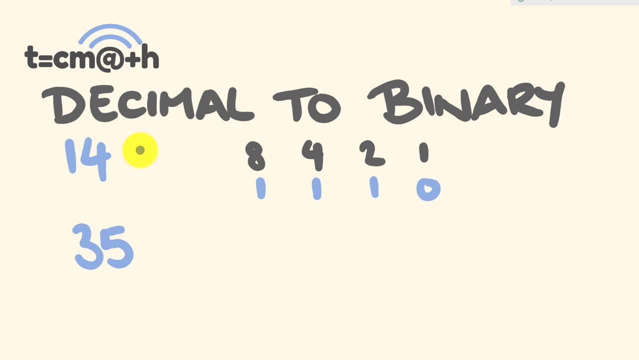 equal to 14.. We don't need this 1 here, So 14 in binary is 1, 1, 1, 0.. For 35, we're going to start doubling 1, 2,, 4,, 8,, 16 and 32.. But we don't need to go any further, obviously, So we're going to be. 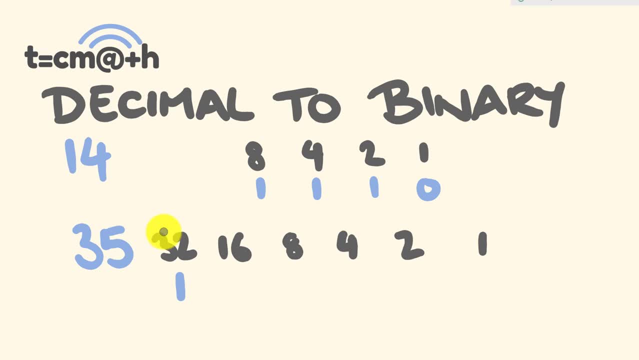 using this: 32.. We always use this first number here on the left. And to 32, you can probably think, OK, we just need to add 3 to it. So 3 can be made up of 2 and 1.. The rest of these numbers: 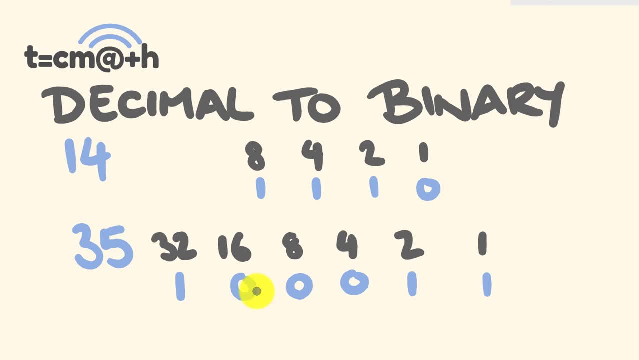 0 underneath. So 35 in binary is 1, 0, 0, 0, 1, 1.. And that's how you convert any decimal number to binary really quickly, really easily. Anyway, tell us what you think of that video And please.